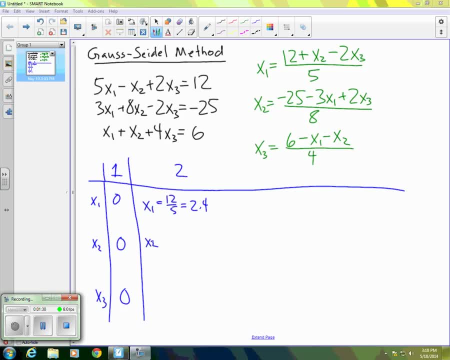 use the green formula up above and to the right. But we now have a new value, of x1 rather than zero, So let's use that new value. So we have negative 25, minus three times 2.4,, which is the most recent value of x1.. The most recent value of x3 is zero, So we 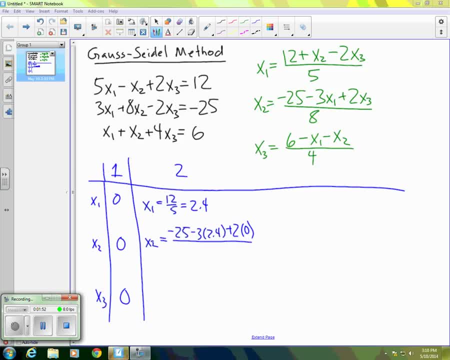 have 2 times 0 there in that spot And we're dividing by 8.. And when we do that, the value we get is negative 4.08 times 1.. Right, This doesn't seem to say actually negative 4.8, but it means 4.. τ is the value we get. it doesn't seem to say actually negative 4. dx, but it means 7.. So we get 4. Street Zelλ 0. and we have 0. And when we do that the value we get is negative 4.08 into 0.. Theta. 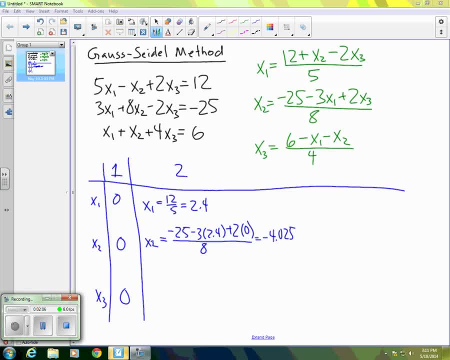 equinox and 0.4.. And when we do that the value we get is negative: 4.. Theta: 025.. So that's our second x2.. And now for our second x3, we again use our equation above and to the right, but we use the most recent values we have for x1 and x2.. So we have 6. 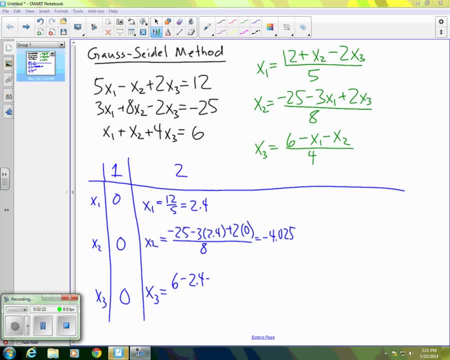 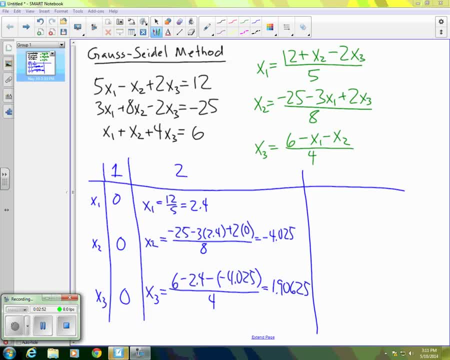 are one negative 3 and 2.. We can see that the x3 is pretty close right now And of course that would make sense because it had the advantage over the other two of using the updated values of x1 and x2.. When we go on to our third iteration, I'm not going to 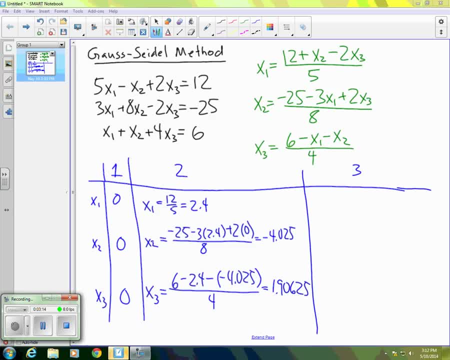 have room to squeeze everything in here, but let me just see what I can fit. So the x1 is going to be 12. plus the most recent x2, so thats from our previous steps that's negative 4.025, and then minus two times our most recent x3. 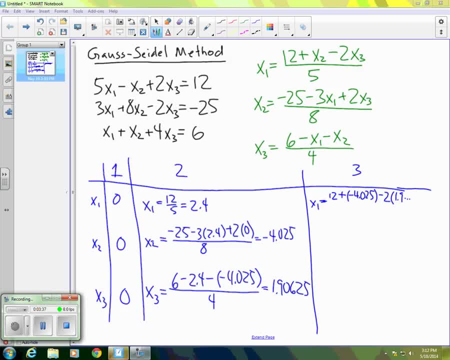 which is the 1.9, da, da, da, and it's all divided by 5 and that comes out to be 0.8325. now, when we go on to find our our third x2, we'll go ahead and use that 0.8325 value that we just obtained. 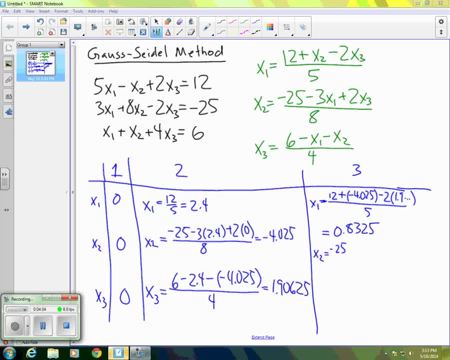 so I have negative 25 minus 3 times 8, or 0.8325, and plus 2 times that value we had of x3, which was 1.9, etc. and that's all divided by 8 and the result of that is negative. 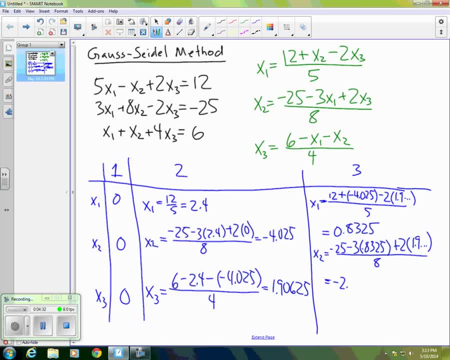 2.96 0625. and in the interest of room here, let me just tell you what we get for x3 this time around. we get 2.0325 uh 203 125. so again, remembering that the actual value of x1, exact value. 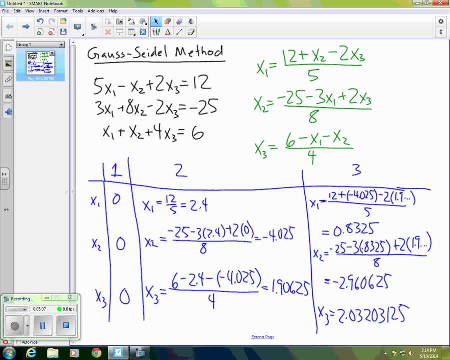 is 1, we're off by a ways there, but x2, the actual value is negative. 3, and you can see we're pretty close, and the x3, the actual value is 2.0, excuse me as two, and so we're quite close there. if we were to go on one more iteration.